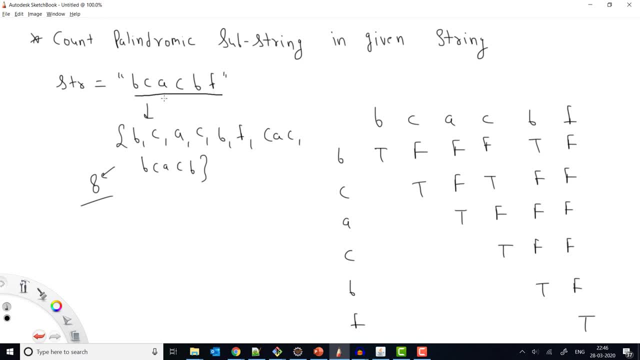 string b, c, a, c, b f, then how many substring, how many palindromic substring we have. So first of all check with the each character. So for the each character we have b, c, a, c, b f, because 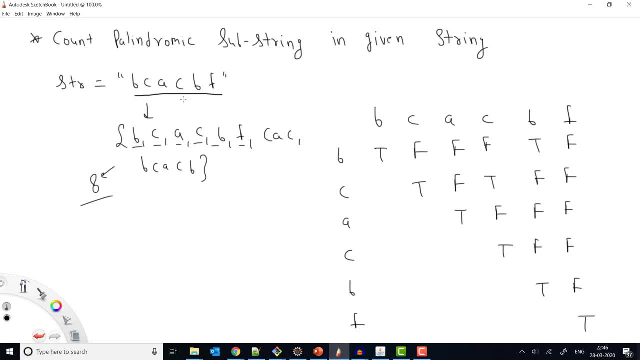 because we have one character, So one character can also have the palindromic substring of the one length, right. So this is possible because if I reverse this single character, this will be same. Now, if you see after that, we have this: c a c. c a c is also a one of the. 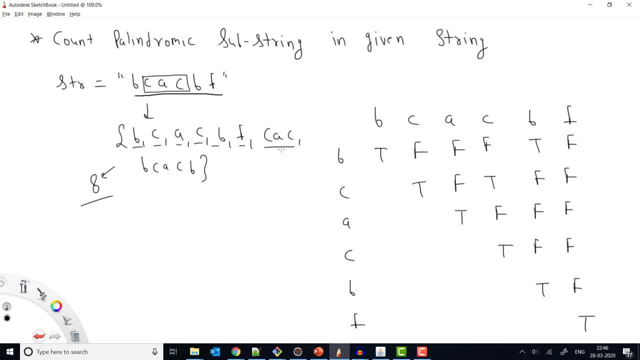 palindromic substring right. So that will be also one of the palindromic substring. Then if you see this one, b, c, a, b, this is also palindromic right. So this we have also written. So it means: 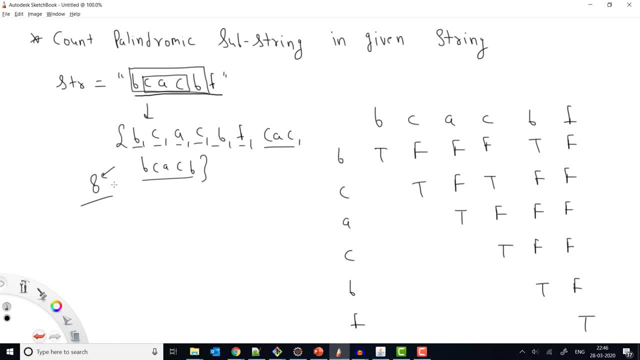 there are eight substring exist which are palindromic or which are palindrome. So my answer should be eight, that in this given string there are eight substrings which are palindrome. Now the point is how you can solve this question right. So basically, before: 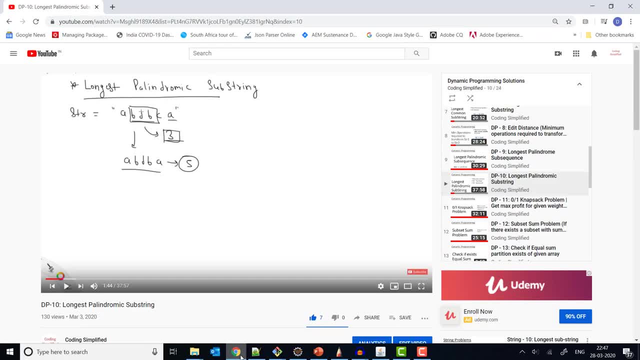 some days we solved a question that what is the longest palindromic substring, right? So in our playlist, if you go into DP 10, we have find out longest palindromic substring. So in that basically we check that what is the longest palindromic substring exist in. 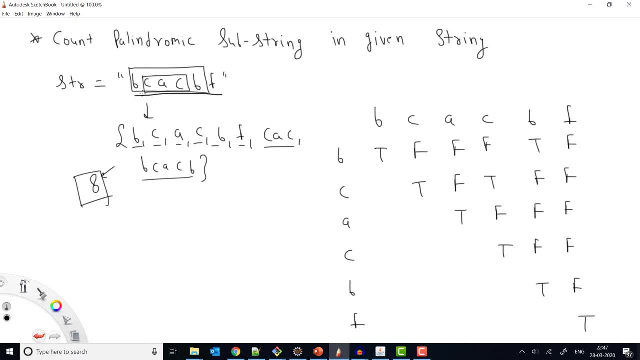 the given string. So like, if you see, in this case, in this case, my longest palindromic substring is 5, right, Because here we have BCACB, which is exactly, which is exactly a palindromic substring, right. 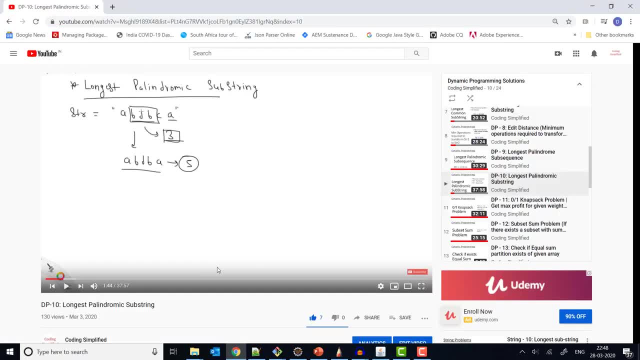 So I would advise you to first go through this video if you haven't seen this video, because to solve our this current problem, we'll basically take the help of the solution of this one right. So if you see in this problem what we do, we basically, we basically solve this. 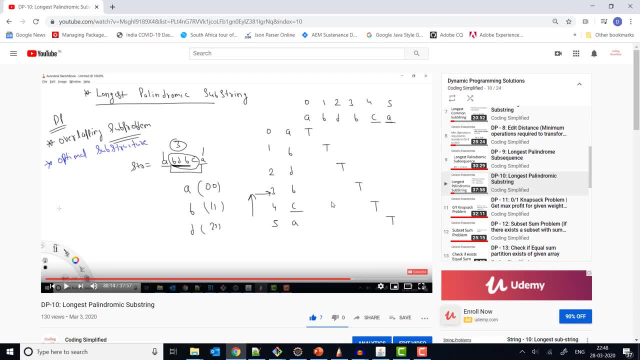 question using DP, bottom of solution, right. And in this we create a 2D array. 2D array with the Boolean values And in this we assign all values to the true. And then we keep on, and then we say: 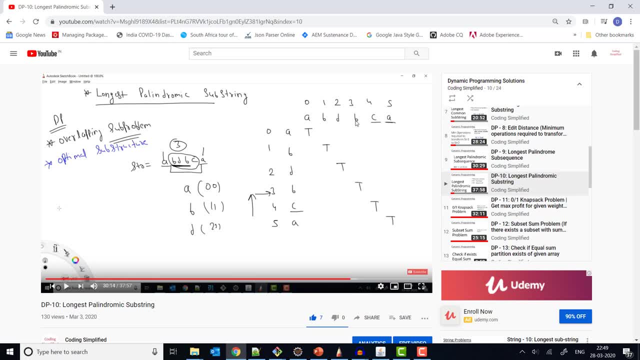 that we start from here and we check that if the, if the characters are equal, if the characters are equal, then we check if the a minus, if a n minus one, and if your matrix n minus one and matrix And minus one. if it is true, then also we make it true, Otherwise we make it false, right? 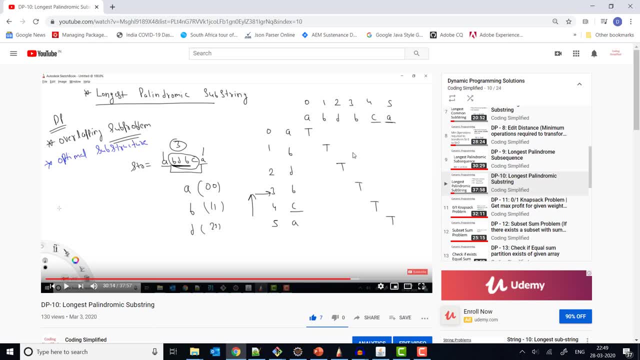 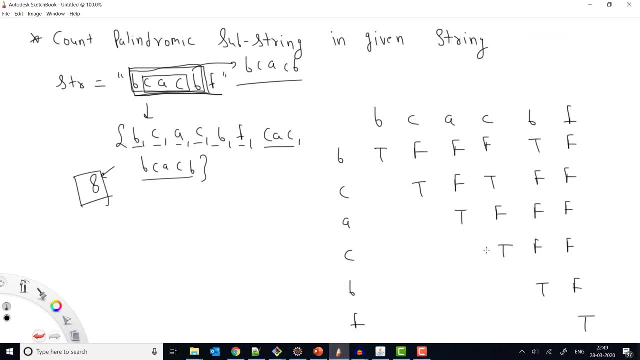 So, when you solve this question, what we need to do, that whenever you have the true, whenever you have the true, then in this case we are getting a one substring right. So let's start from here: how we fill this value. So, basically, this is the exactly same. 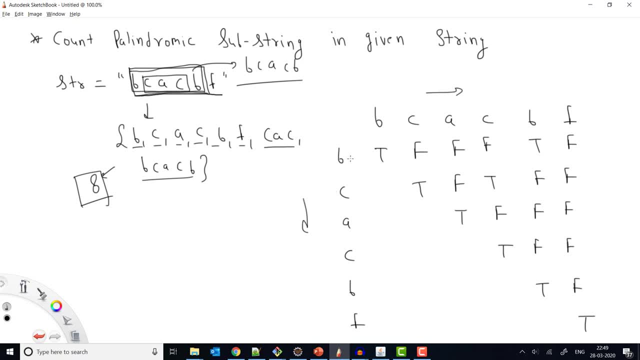 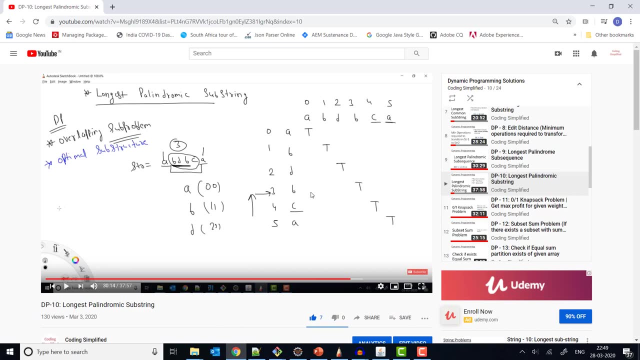 string we have written BCACBF And here also we have written BCACBF, right, And guys, I will not explain that, how I am filling all these values and all that thing. That is why I'm saying that if you haven't seen this video, if you haven't seen that how we are filling this value, 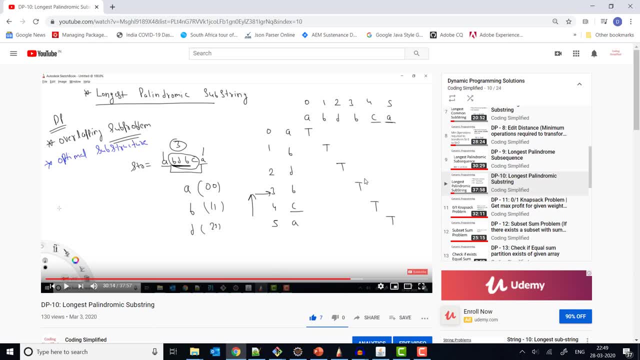 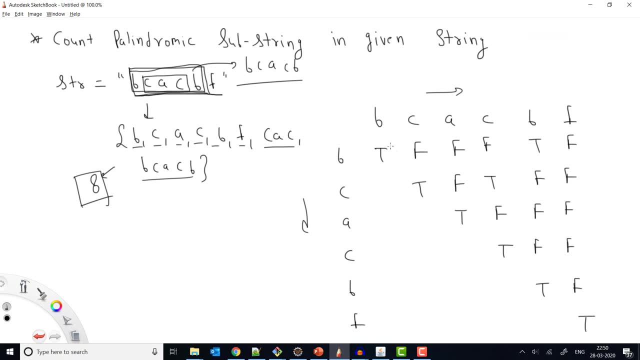 please fill this value right. So now I'm assuming that you have seen this video, So let's proceed further. this one, right. So in this video, what we do? first of all, we basically assign all these diagonal values to true. So diagonal values means, because each string has 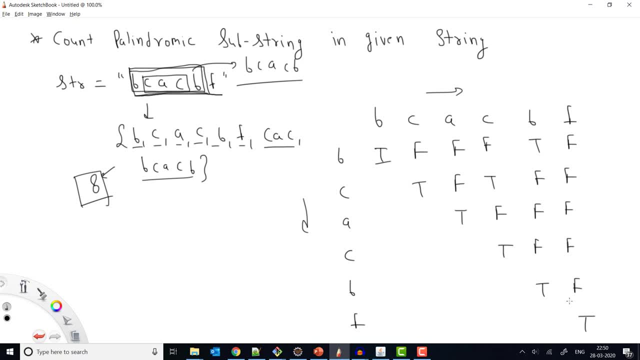 they are of length one. So it means they are of length one. So it means they are of length one. So we are at least having the substring right Now. what we do, we basically start from here and we check that this is I and this is J, right, So basically I start from here to here, like this: 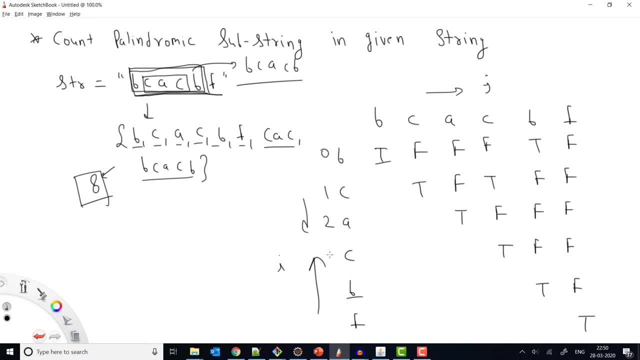 one. So basically, if you say this is 0, 1,, 2,, 3,, 4,, 5, and here I have 0, 1,, 2,, 3,, 4,, 5.. So 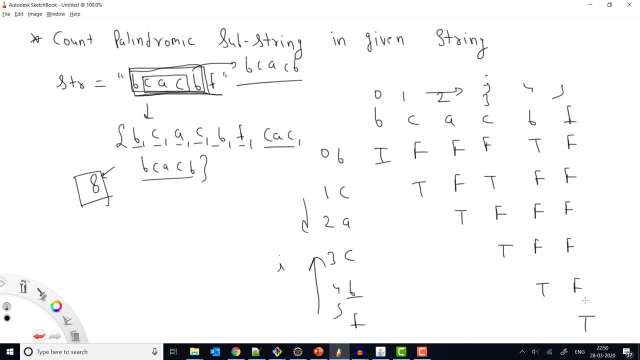 basically for this last one- I need not to check because this is only one. Now I start from here, from the last row, the previous row, And I keep on going to the top. So this is my I and my J will be of the I plus 1.. My J will start. 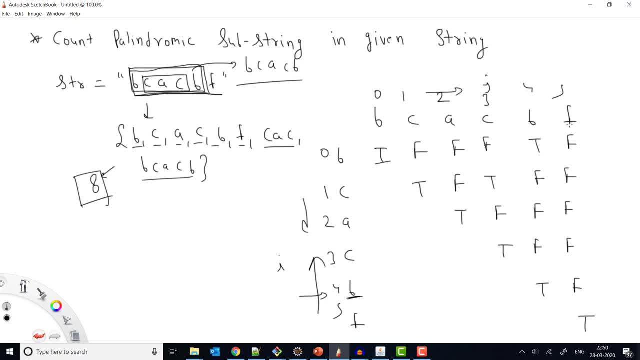 from I plus 1. And I check that if these values are equal. if these values are equal, then I check that. if values are equal, then we only check if the previous, if the previous N minus 1 and M minus value is also true. If it is true, then we feel that true. right, This is how we do. this is how 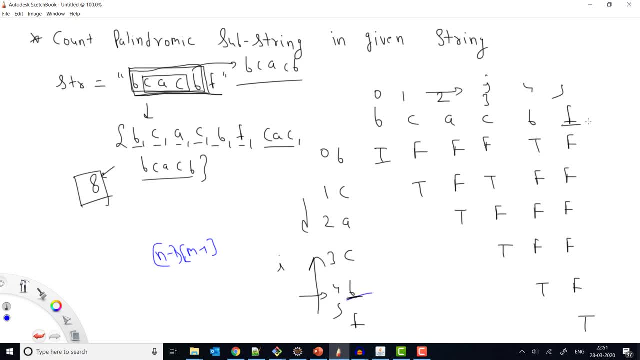 we solve. So like check first of all this one: B and F, it is equal. no, So you. so we feel as false. Now we will check this row Now: C and B, C, because our J will always be. 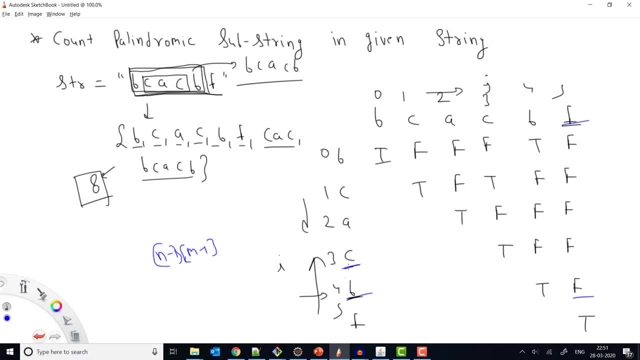 start from I plus 1.. So my I is 3.. So my J will be at 4.. Now C and B are equal. no, It means this is false. Now C and F are equal. no, This is false, right. So here we have this one, and here: 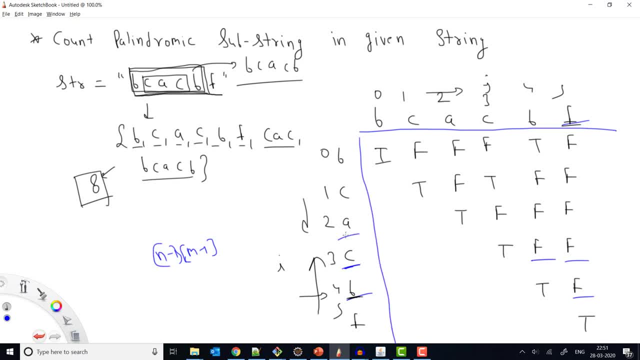 we have this one Now. check for this: A, A and C are equal- no, A and B are equal- no false. A and F are equal- no false right Now we check for this: C. C and A are equal- no false. C and C are equal, yes. So if C and C are equal, 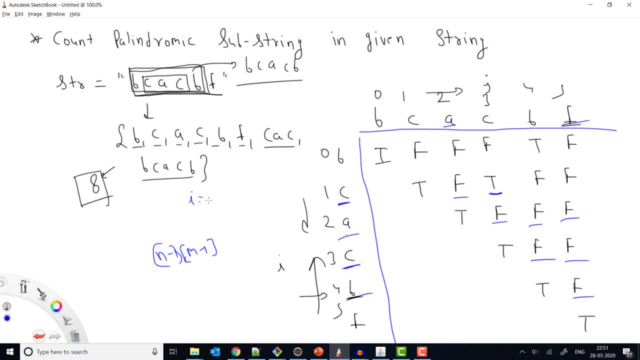 it means? what is the value? My I is, my I is 1 and my J is 3.. So basically I check if N minus 1 and M minus 1 is, also if N minus 1 and N minus 1 is also true, right? So basically we check with the 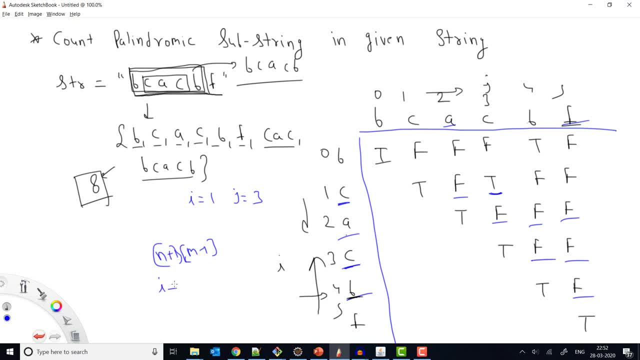 N plus 1 and M minus 1.. So basically I plus 1 and M minus 1.. So basically I plus 1 and M minus 1.. This one is J minus 1.. So it means I is 2 and this is also 2.. So what is 2, 2?? 2, 2 is this one. So this is also. 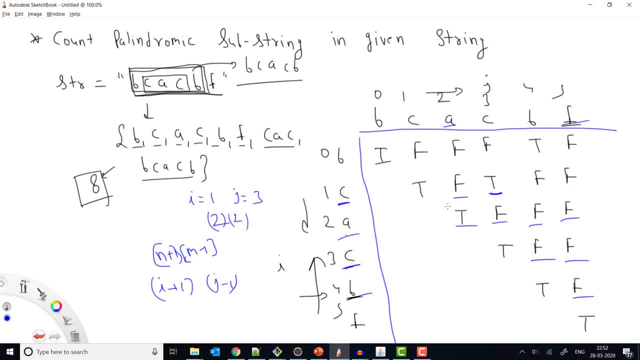 true. So if it is true, then it means there exists a polyぐlomic substring. So if it is true, then all we make is true. So now we have true, right Now. C and B are equal. no, false, C and F are equal. 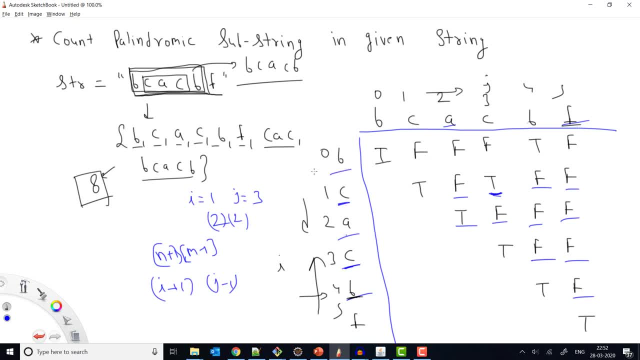 no false. Now check with this one: F, F and B. sorry, B and C are equal- no false. B and A are equal- false. B and C are equal- no false. B and B are equal- no false. So it is true, right. So now. 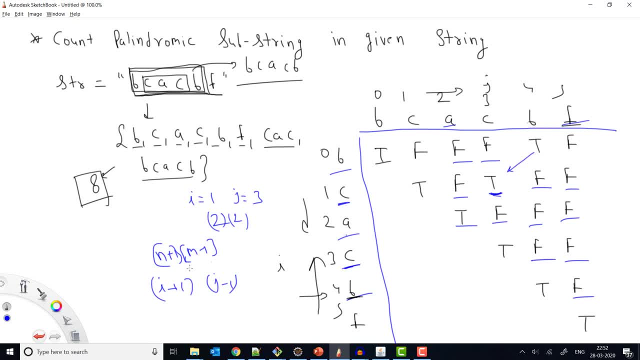 equal. if b and b are equal, so we check with a diagonal value, means i plus 1 and j plus 1. so this is true. yes, so if it, if it is true, it means we will also set it true. and at the last, b and f. 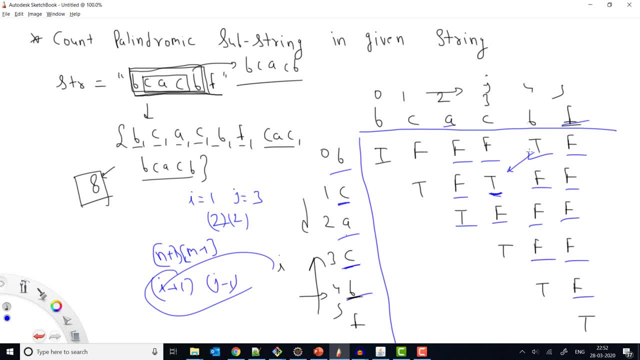 are not equal. so it is false right now. what now? if you observe here, whenever there is a true, then we are getting a palindromic substring right, because these were the single, single substring. so here we are getting true right. and when we go to this true here, when we go to this true here, 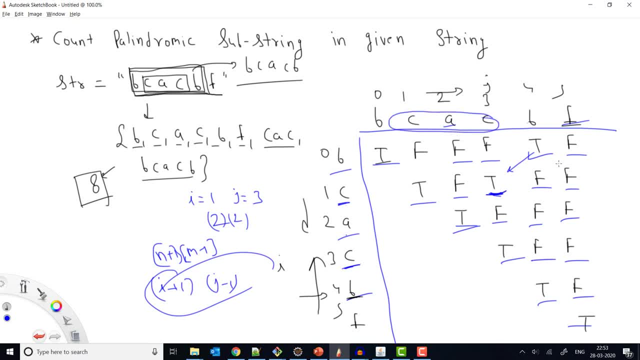 then also there was a substring cac, and when we go true here, then also there was a substring which was palindromic, right. so it means, when we fill this value, then we'll will be, then we'll be getting true only when we are getting a palindromic substring right. it means what you will do, that 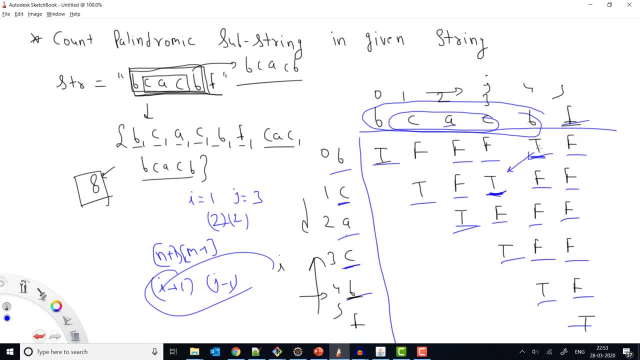 whenever you will, whenever you will achieve a true, then i will basically increase the count. so at this starting my count will be of zero and then whenever i will keep on filling the value right. so basically i can start my count with this value: one, two, three, four, five, six, because i know that the so basically the string length. so string length i can start. i. 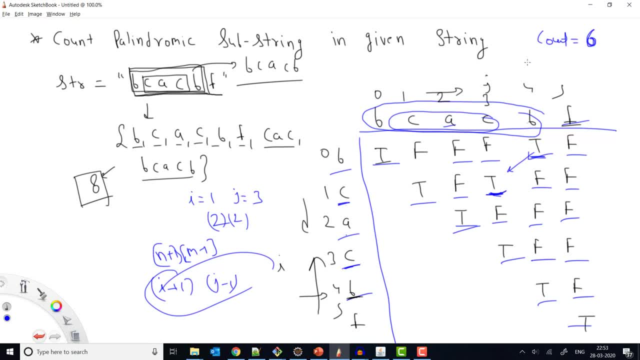 can installize with this, because i know that there will be. there will be at least one palindromic substring of length, one right. so basically i can start the str dot length right now whenever i'm filling the value and whenever i am getting true then i will increase the value. so at the starting, 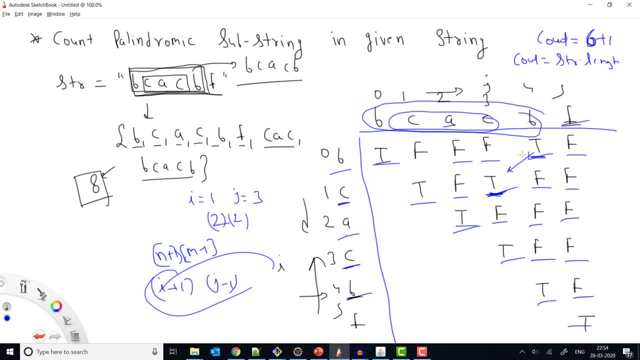 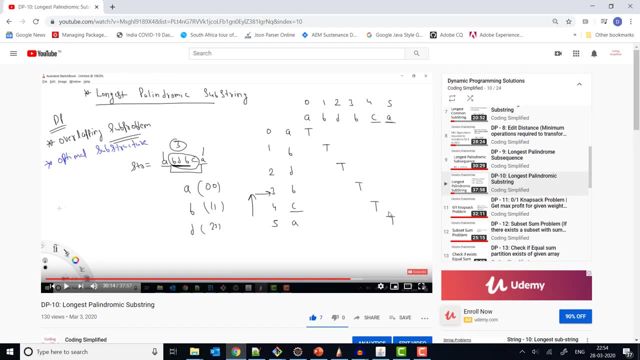 it was six. then i got the true, here i will plus one. then i got here, i will add plus one. so at the last my answer will be six, right? so this is how, basically, i'll get the value right and then how you are filling this value and how that. so basically, you can basically explain, you can. 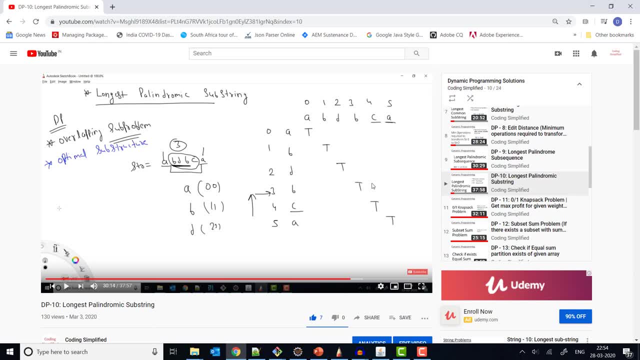 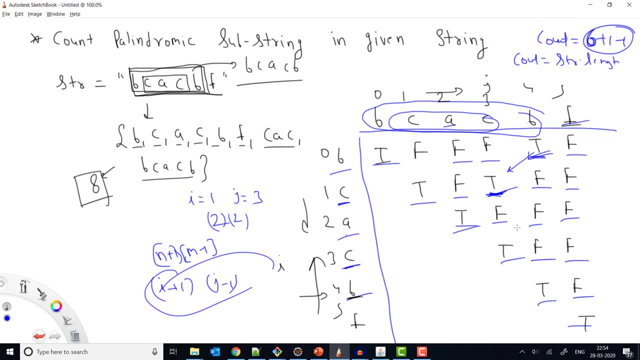 basically, uh, check from here and once you get the solution of this one, then you can easily check this one. that whenever we are filling the value, you can easily basically convert this solution into that one right. so this is how we basically get our solution now. if you want the time complexity, so my time complexity will. 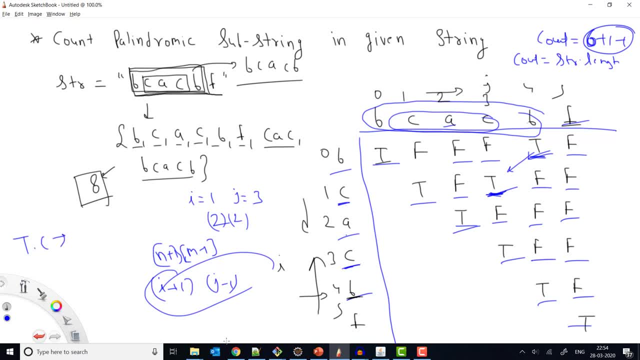 be exactly with the same, as you are getting this solution longest panadromic substring right. so this will be the same time complexity. so please check from there and then you can easily check it. now let me show you the code as well, so that you can get it better. 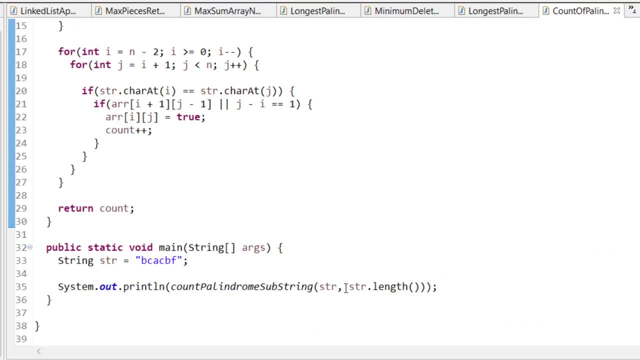 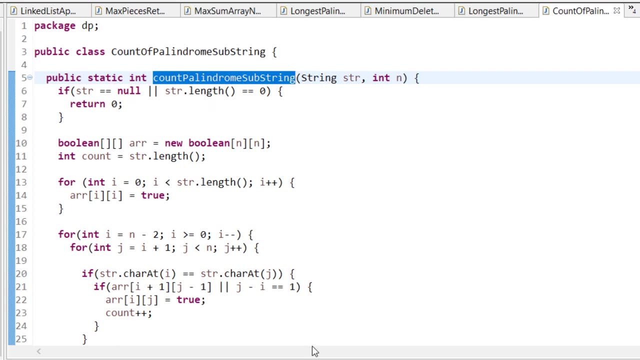 so here is my string and here is my here this is how i'm calling the function count palindromic substring, where i'm passing the string and str dot length right now. uh, now here is the negative cases, that if my string is null or if my string length is zero, 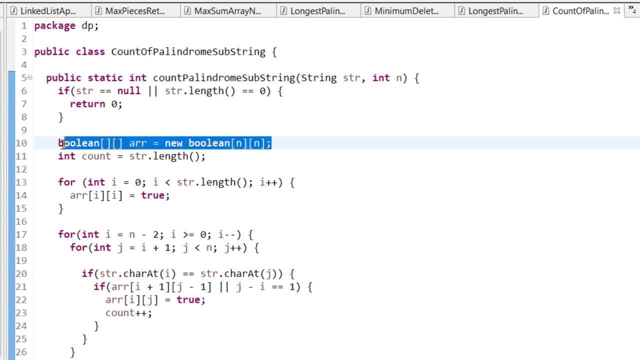 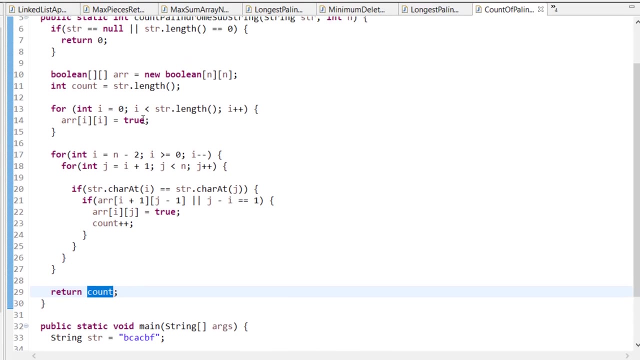 then i return the zero. else i basically initialize a boolean array, boolean 2d array and the. at the starting my count is equal to string length, right, so this is basically the count of palindromic substring. at the last i will return basically this count. right so at the starting, because i know that. 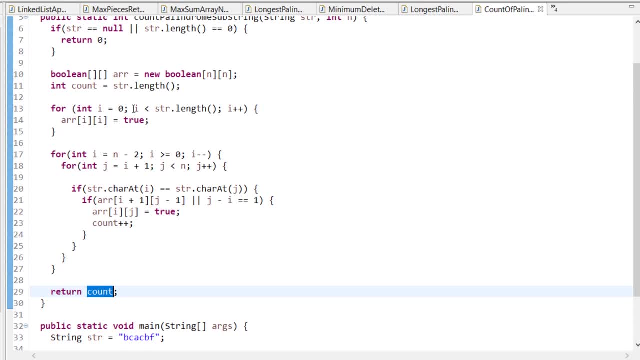 this diagonal, i am filling all the values true, so at least it would be the string dot length substring right. why this is because at least there will be of one length string equal to the string dot length. now, when i'm filling this value, now, whenever i get the true, whenever i get the true, 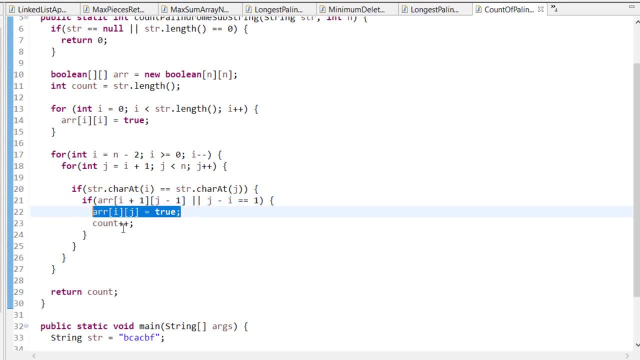 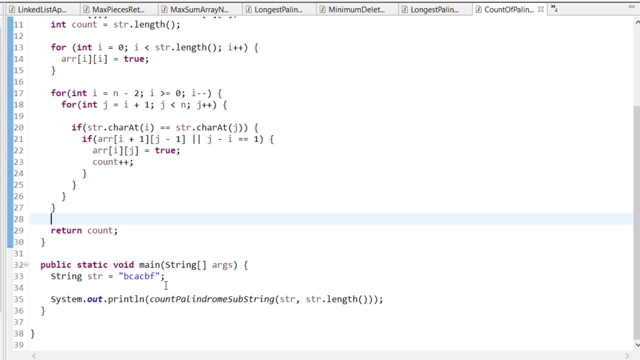 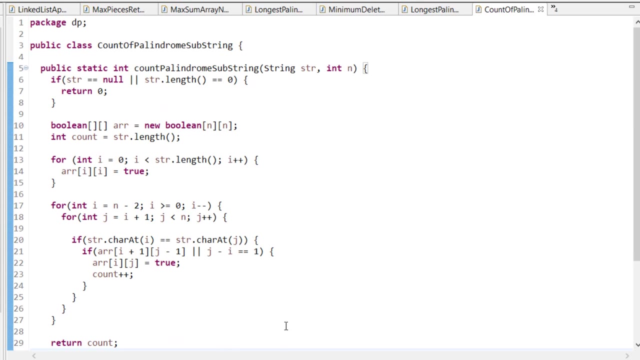 then at the same time i increase the value of the count right and at the last i will return the count right. so this is how we basically can get that- how to find the palindromic substring count right. so that's it, guys, about this video. if you have any doubts, then 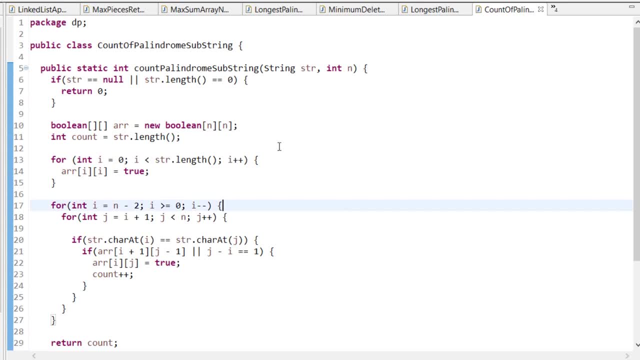 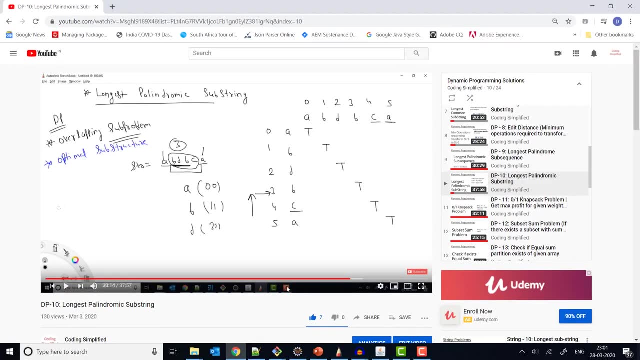 please write in the comment section. i will also post the source code of this into description section, so if you want, then you can also get it from there. and similarly i will also put the link of this video so that you can get it better. so thanks, and if you have liked the video, 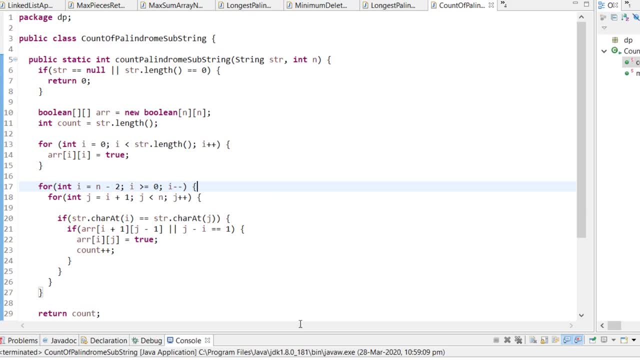 then please like it and subscribe the channel for more such videos. thank you. 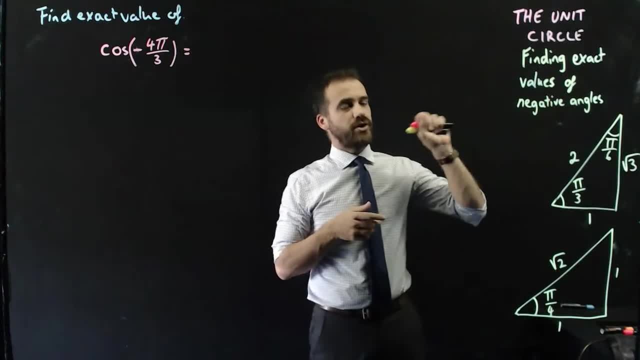 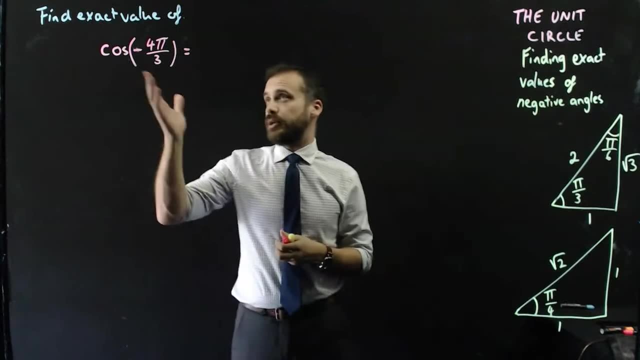 Alright, we're still finding exact values here. This time we're going to find values of negative angles. Now this is actually really easy. It's the same as before. You've just got to consider one little thing. So we're going to find the exact value of cos negative, 4, pi on 3.. 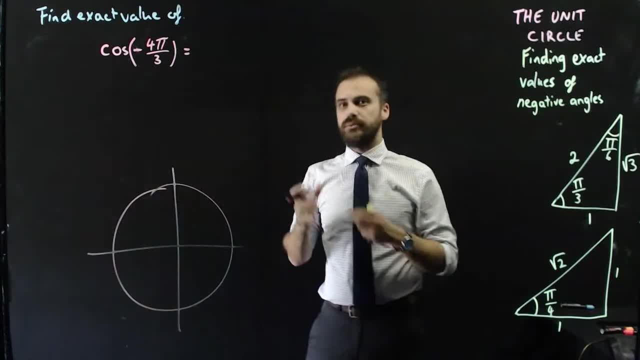 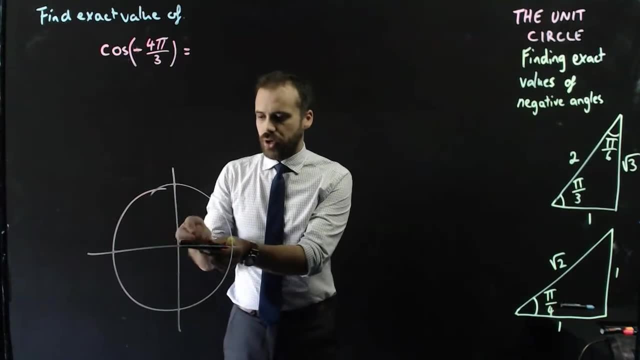 I'm going to draw a unit circle, because I always draw a unit circle when I'm doing this stuff. A negative angle. A negative angle just means that it's moving clockwise, Not anticlockwise like all of the other angles we've done.